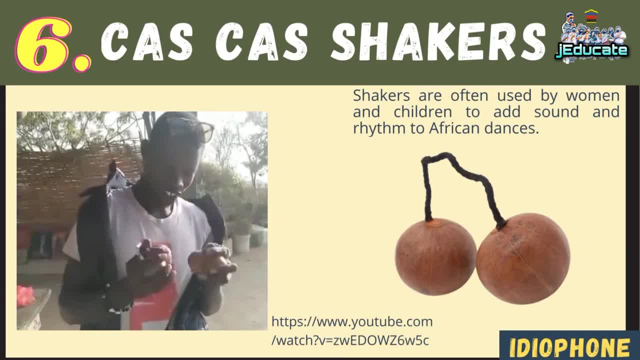 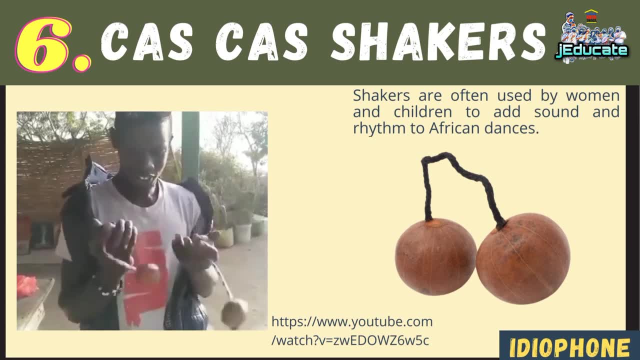 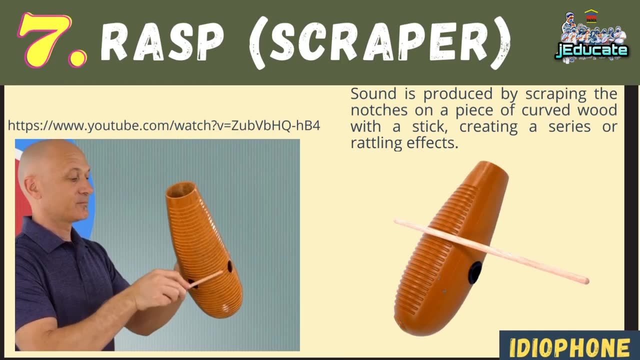 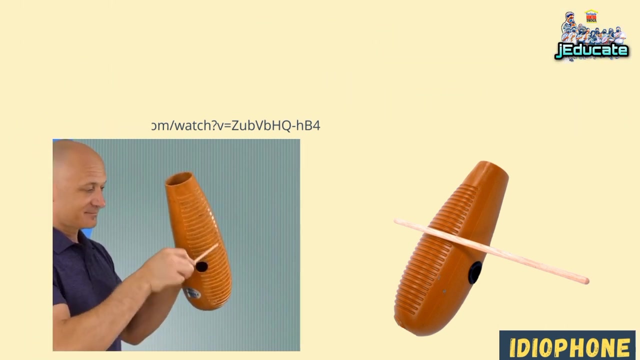 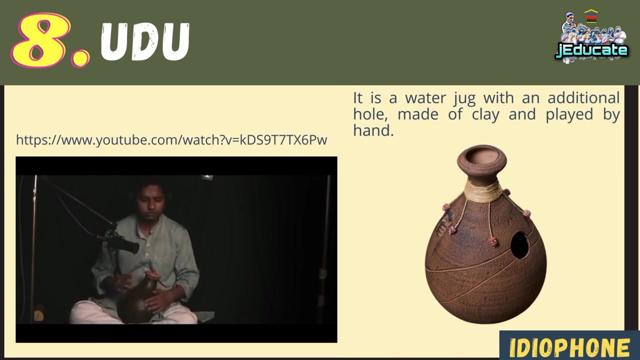 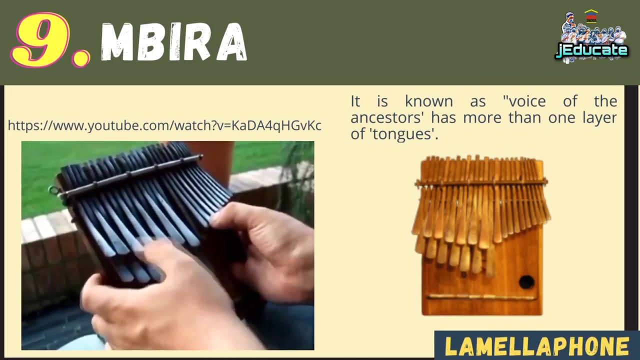 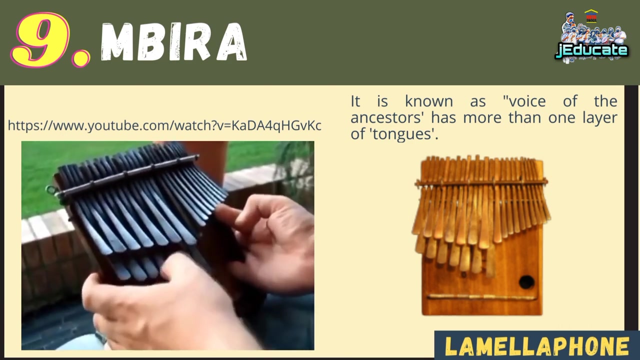 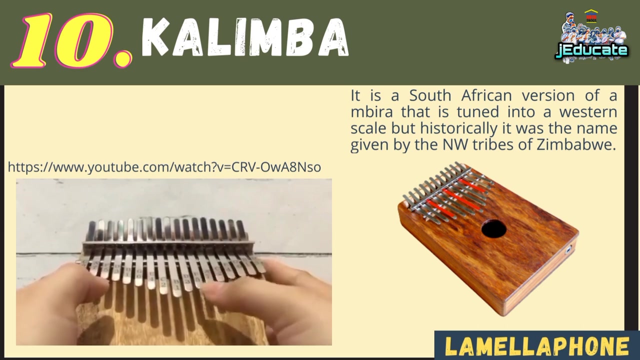 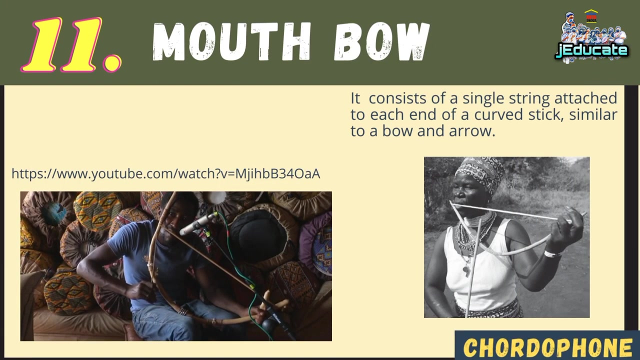 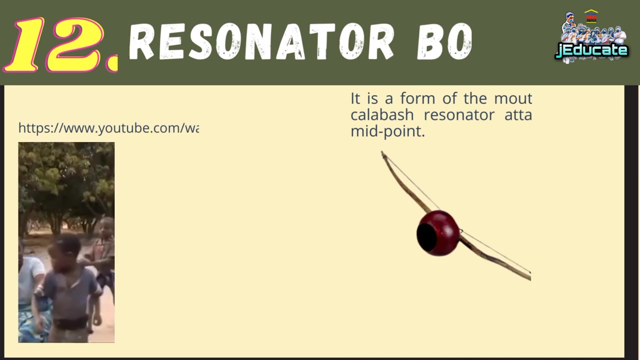 Number 6. Sawz Sawz Shakers Number 7. Rasp Scraper Number 8. U-Do Number 9. Mbira Number 10. Kalimba Number 11. Mouth Bow Number 12. Resonator Bow. 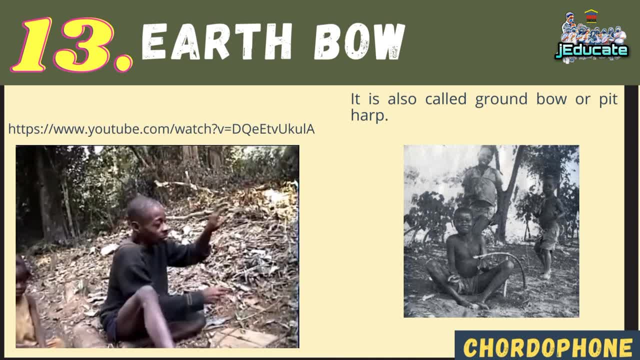 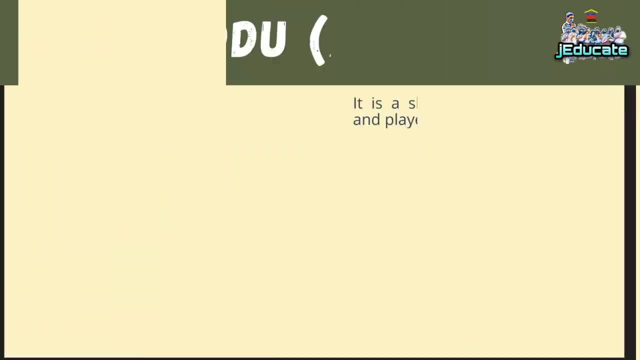 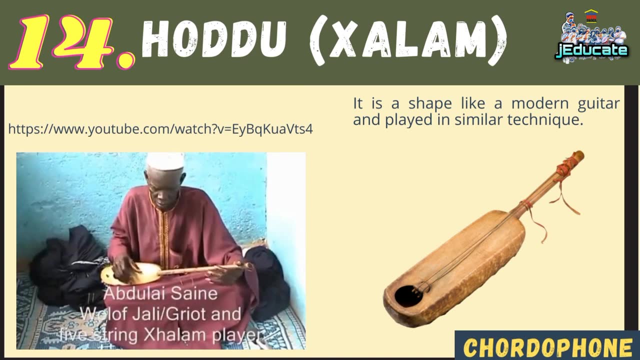 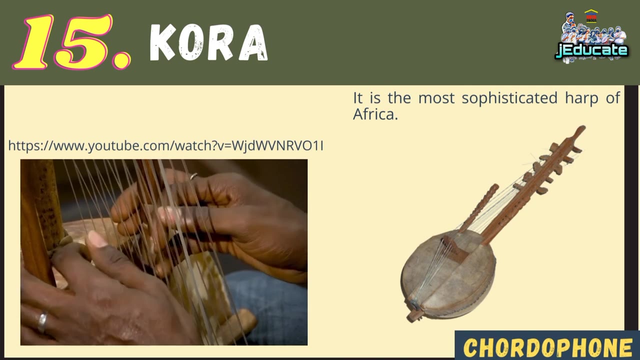 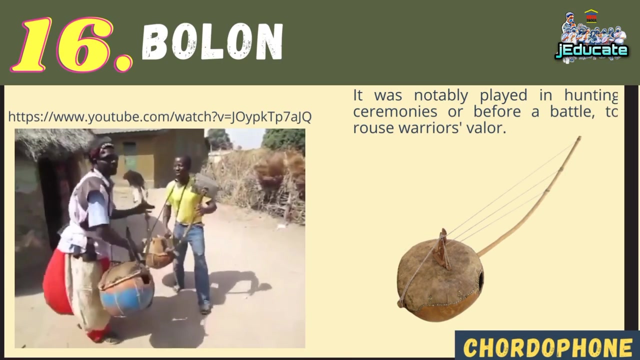 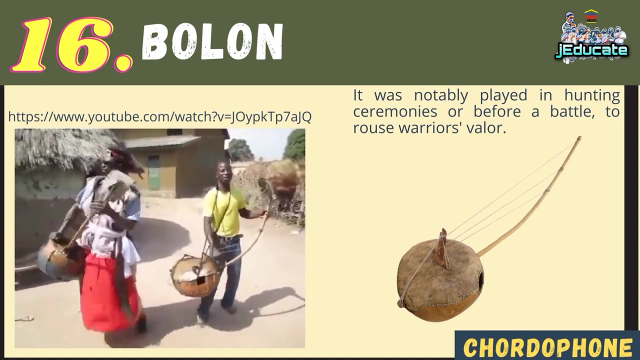 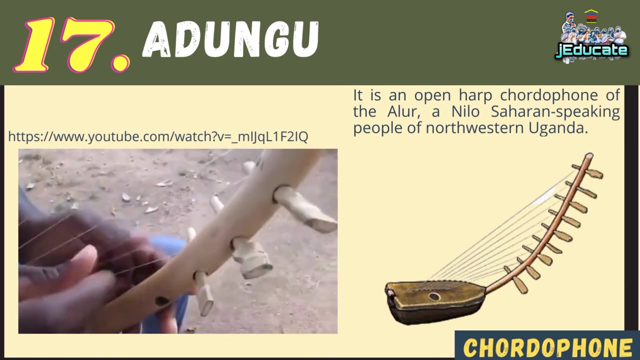 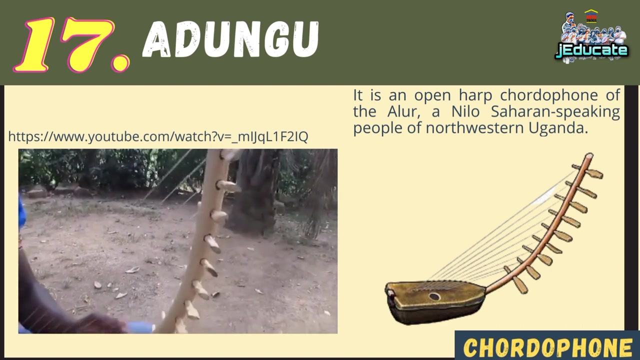 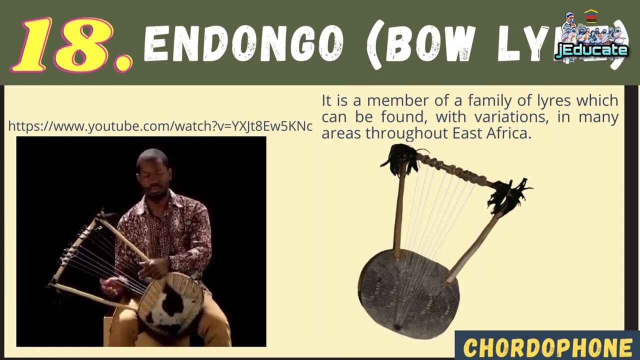 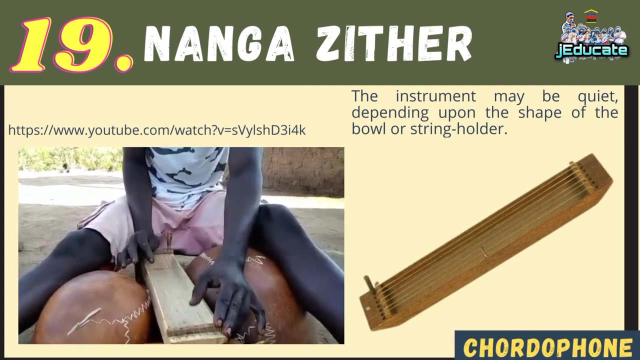 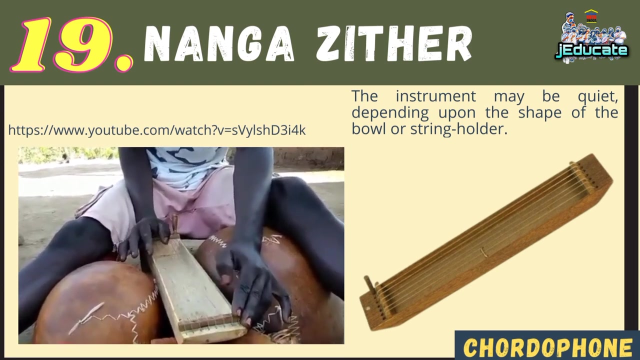 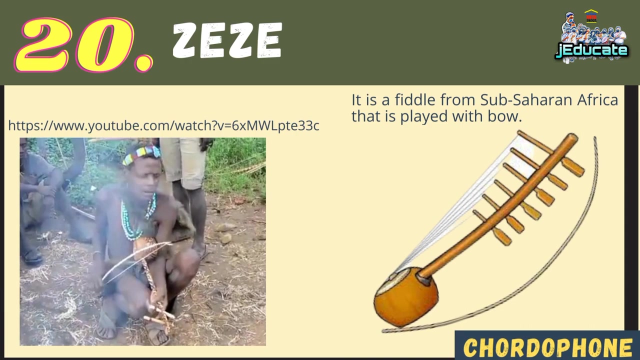 Number 13.. Earth Bow, Number 14.. Hadu Number 15.. Korah, Number 16.. Belonging number 17 a, dungu number 18 in dango bow, liar number 19, nanga zither number 20 zeze.